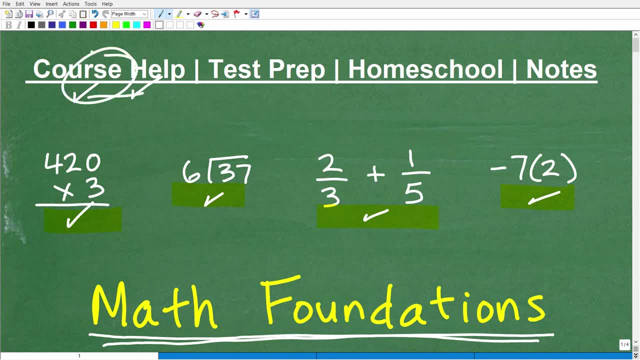 So if you happen to be studying any of those courses, I could definitely help you prepare and pass those courses if you're taking any exam that has math on it. So, for example, the GED, SAT, ACT, GRE, GMAT, ASVAB, ACCUPLACER, ALEKS exam, CLEP exam, teacher certification exam. 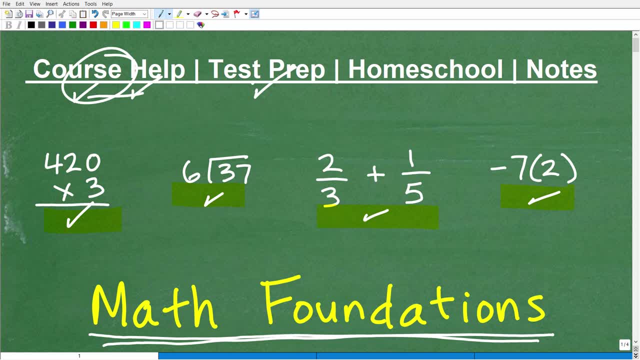 You get the idea. I can help you prepare and pass those exams. Of course, each one of those exams that I have, as I said, has a math section, So somebody thinks math is pretty important. If you homeschool, I have a very comprehensive homeschool math curriculum. 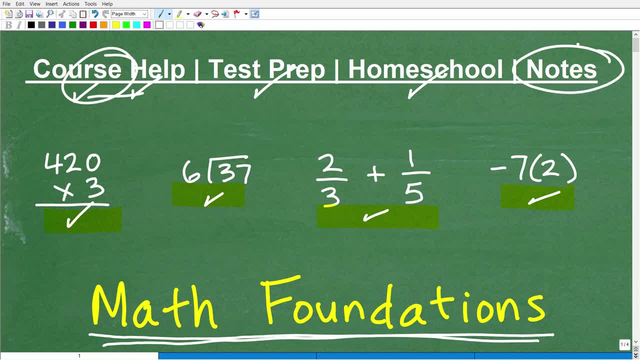 And if you don't have any math notes, don't stress out. I have math notes that you can use. I'll leave links to those notes in the description of this video as well, But you need to start taking effective math notes. This is really the secret to being successful. 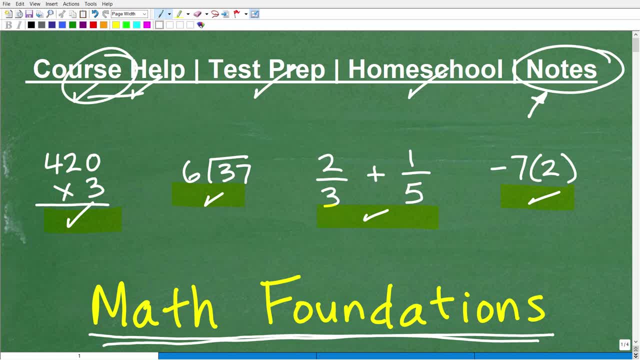 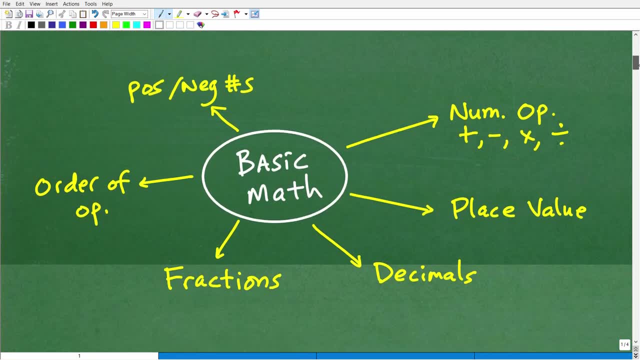 And mathematics. So let's get into basic math skills that every adult should have, And I'm just going to kind of give you a quick summary of things that I teach in this basics math foundation course that I just constructed. But let's just kind of start over here. 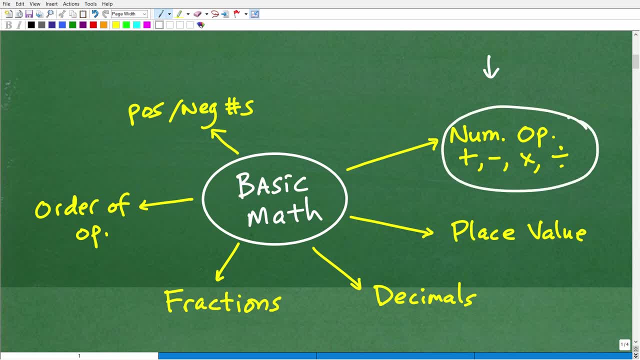 And the first thing is number operations. Everybody should be able to have basic arithmetic skills. You should be able to add numbers, subtract, all without the aid of a calculator. Now you should know how to use a calculator as well. I'm talking about good old-fashioned arithmetic pencil and paper. 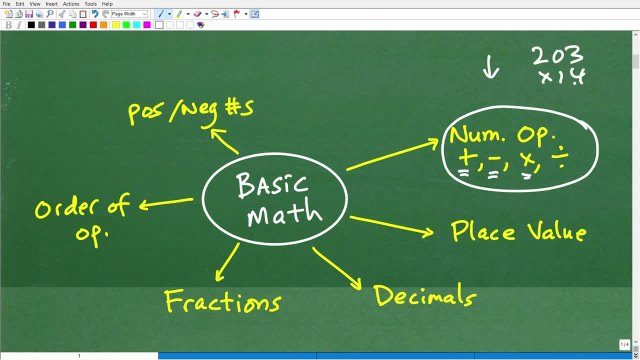 If I gave you 203 and I said, multiply that by 14, in other words, do a problem like that or give you like a division problem 6 into 37, go ahead and do that and give me the remainder. This is the kind of stuff I'm talking about. 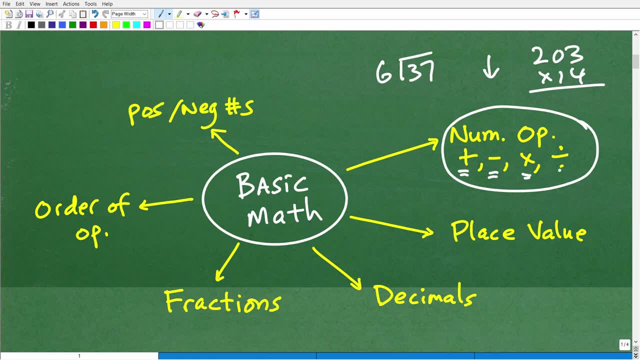 So basic number operations- adding, subtracting, multiplication and division, All right Again, arithmetic- things that we learned way back in, you know, elementary school. But the further we get away From elementary school and basic math and the more dependent we get on calculators, these skills get rusty. 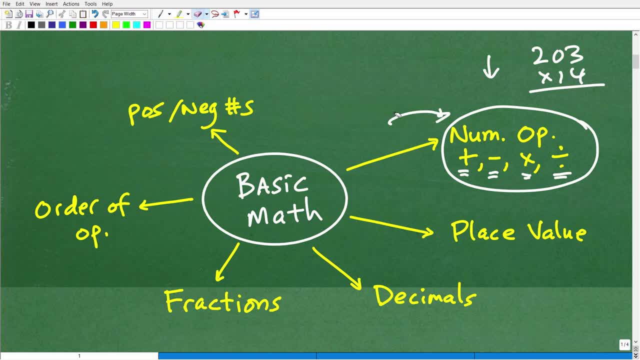 But it's really critical that you still know how to do this. do these basic number operations, because this stuff is also in algebra, Okay. So the next thing I would say is place value, Okay. So what am I talking about there? 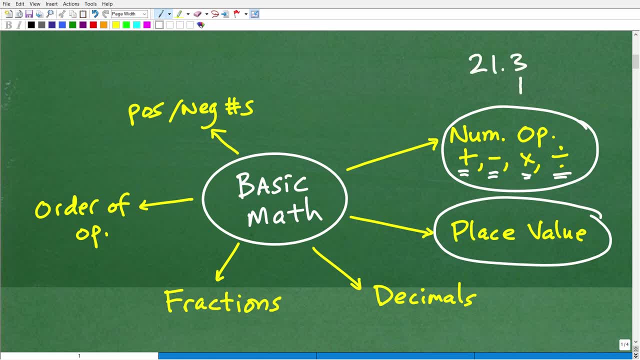 So if I look at a decimal- 21.3, we're talking about the tenths place and understanding decimals and place value. This is very important. So you know when you see a decimal, you understand what place value that represents, et cetera. 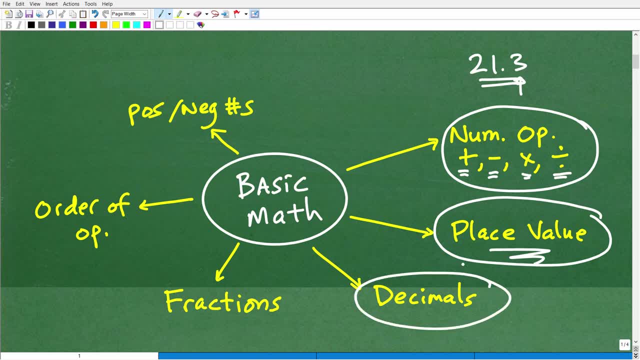 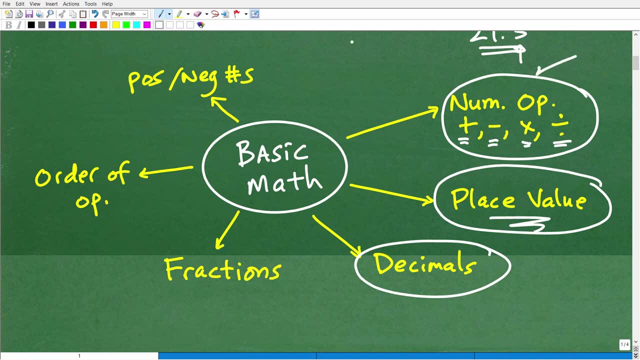 So that's what place value is, And that leads us into decimals. Okay, So now that when I was talking about number operations, I'm talking about basic, whole numbers, you know, for example, 114 times 3.. But what about 114.7 times 3.2?? 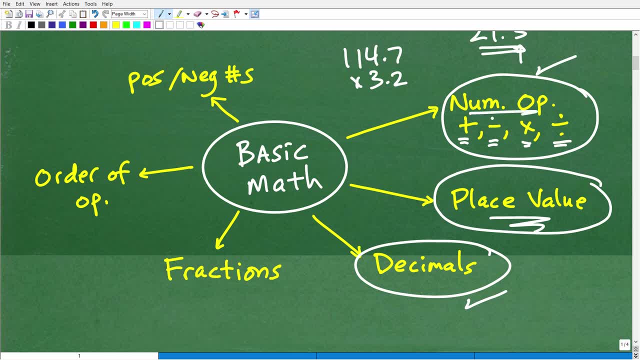 Well, that's decimals. Okay, So you're going to need to know how to do number operations with decimals. This is a little bit trickier And that's why you want to kind of go in this particular order. So you know, a lot of us kind of remember that and we're like, oh boy, I remember doing decimals, you know. 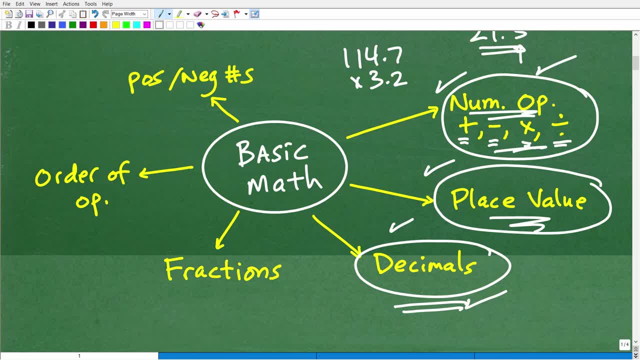 And I would say today: okay it's. you know you need to know this stuff, But if you had a calculator handy, you should be able to just use your calculator. Don't feel guilty about using your calculator. However, don't think that your calculator is a substitute for you not knowing how to do this by hand. 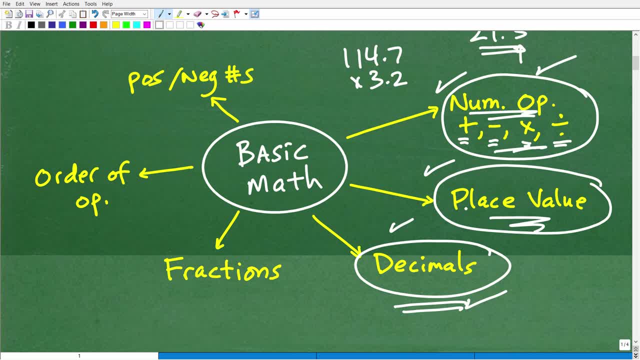 Hand basic arithmetic. Okay, It's still very important that you can still do this stuff. All right, That leads us to our next basic math topic, And that is fractions. Okay, Fractions- critical. Most people do not know fractions as well as they think. 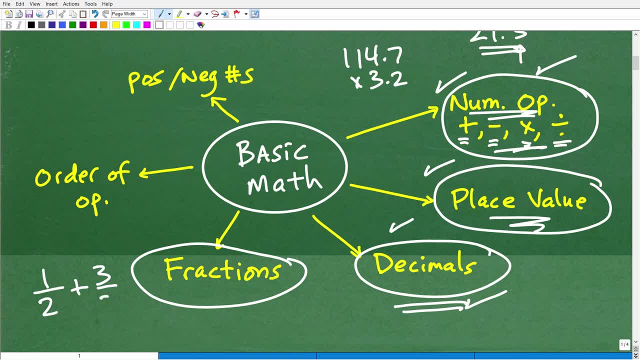 Of course, if I give them a simple problem, one half plus three halves- they can go. oh, I can do that, No problem at all. But if I give you a much more challenging fraction, then it gets more interesting, Okay. 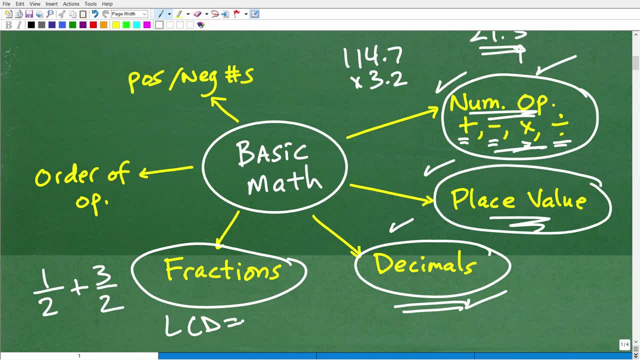 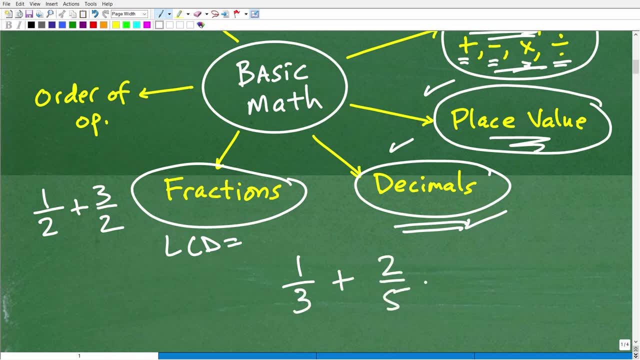 Most people can't tell me exactly How you find the LCD. If I give you again one third plus two fifths, most you could be like, oh, the LCD is 15 and you'd be correct. But how about 32 and 504?? 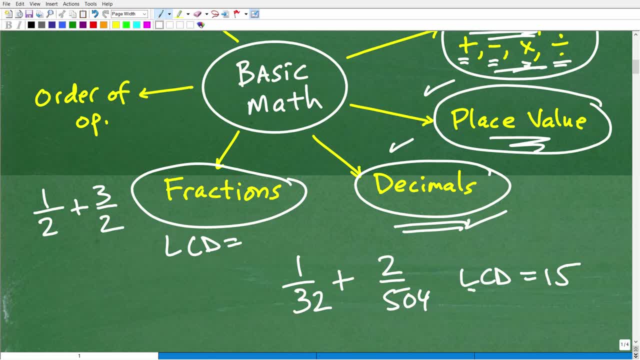 If those were the denominators, this would be much more challenging to find the LCD. So again, all these things that you know, you want to know is not just the basic stuff. Don't get a false sense of confidence. Be like, oh, I can handle. 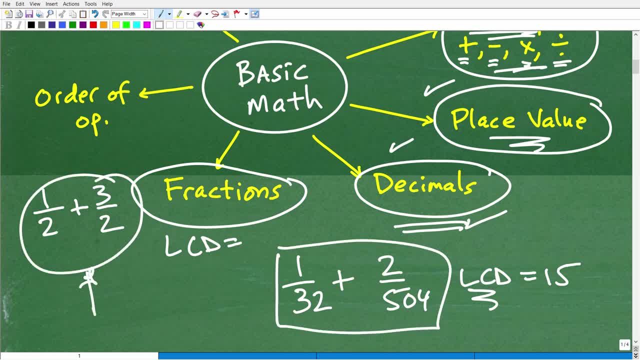 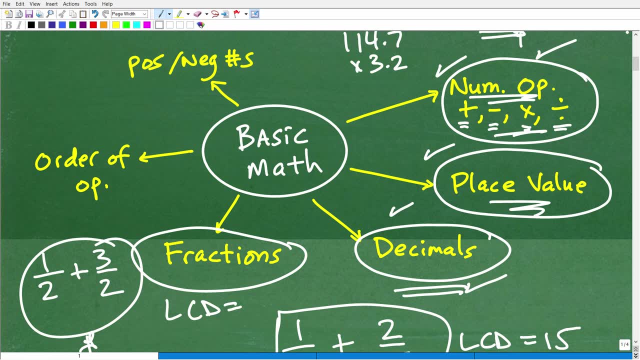 I can do fractions, because I could do problems like this, But what about a problem like that? Okay, So this is what I'm talking about: Really upping your basic foundational math skills, All right. So fractions are very, very important. 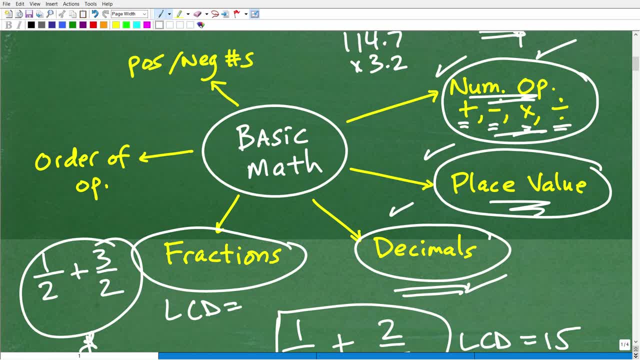 Again with fractions. you're going to be doing number operations, The number operations. with fractions, You need to know how to add, subtract, multiply and divide. Now I want to say one thing: I cover a lot of this stuff informally in my YouTube channel, in my pre-algebra playlist. 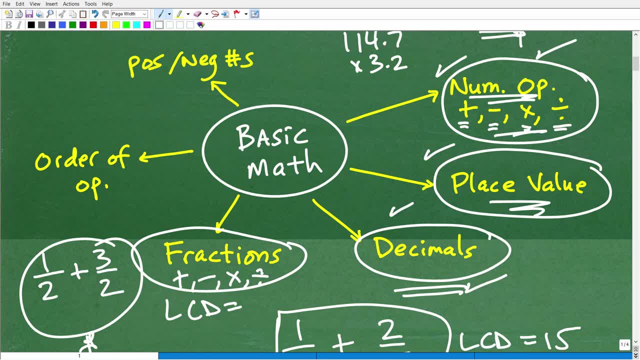 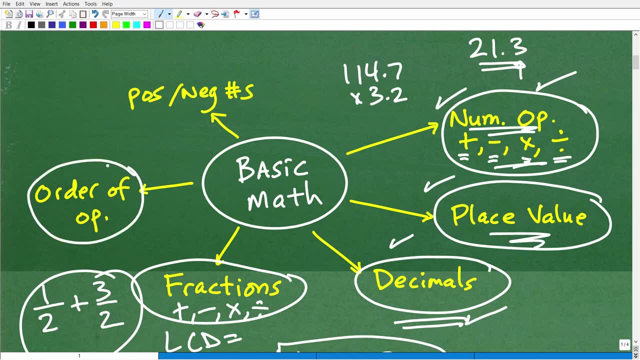 So I have tons of videos on this kind of stuff. This math foundations course is more formal, full kind of instruction on this. But let's continue on. The next thing I would say is like the order of operations. This is this little acronym: PEMDAS, P-E-M-D-A-S. 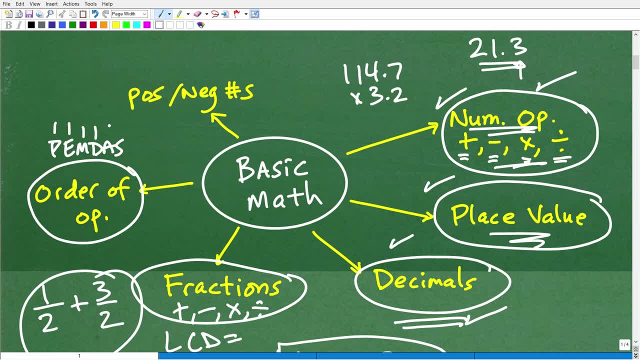 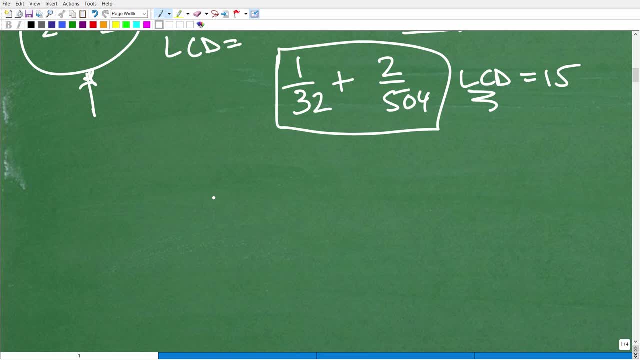 Now there's an old saying that says: please excuse my dear Aunt Sally, but this means something, And what it means is how we deal with a number or a numeric expression. So, for example, if I had two Times seven minus ten divided by three over let's say six minus eight squared, 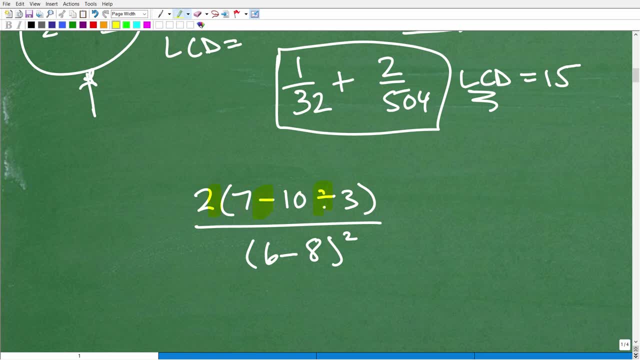 OK, I have a lot of different things going on here. I have multiplication, subtraction, division, subtraction and a power and division. So what is the order? I do this problem? Because I can do, I can do these number operations in various orders. 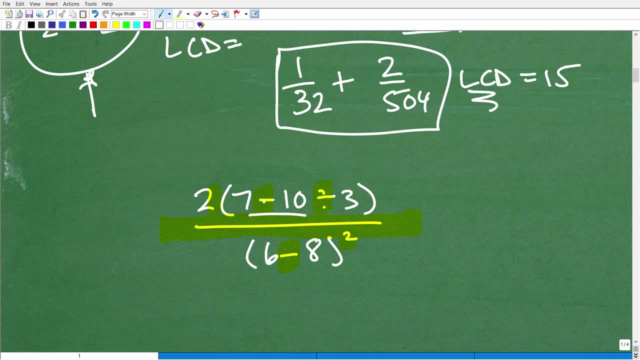 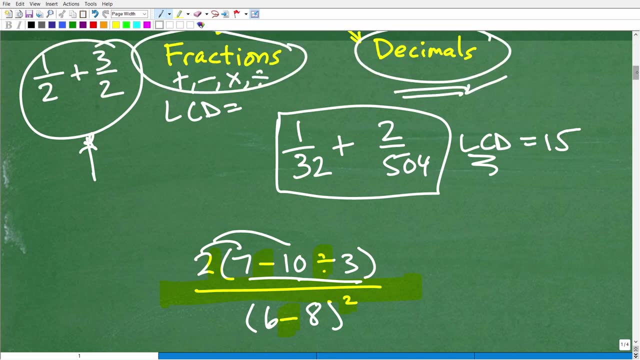 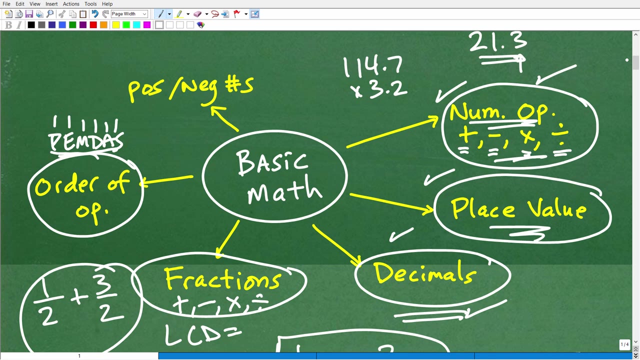 I can subtract here, for example, first, or maybe I can divide first, All right, Maybe I can do Multiplication first. So the way, the order you do this, a particular problem, is going to directly affect whether the problem, the solution is right or wrong. 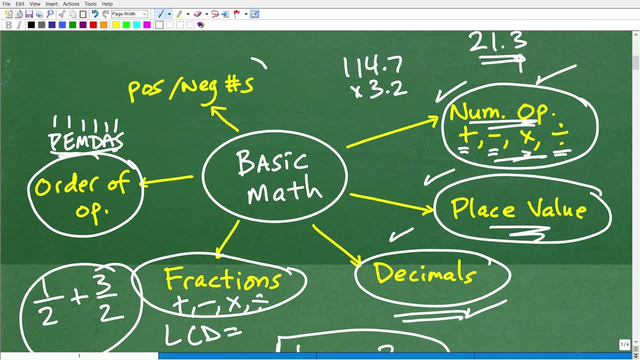 OK, this is very, very important order of operations, And that would bring me to the last thing I'm going to talk about, And that is positive and negative numbers. OK, so we can have positive, negative numbers, You can have positive and negative decimals. 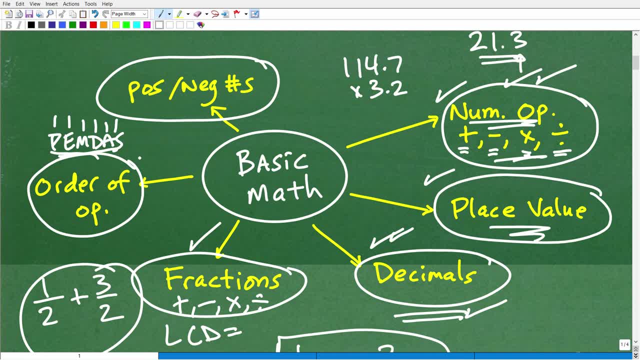 You can have positive, negative fractions, OK, then you can pull those all together And some big numeric expression. So you're going to be doing the order of operations with you know. you can have positive, negative fractions, decimals, all kind of you know put into one big pot. 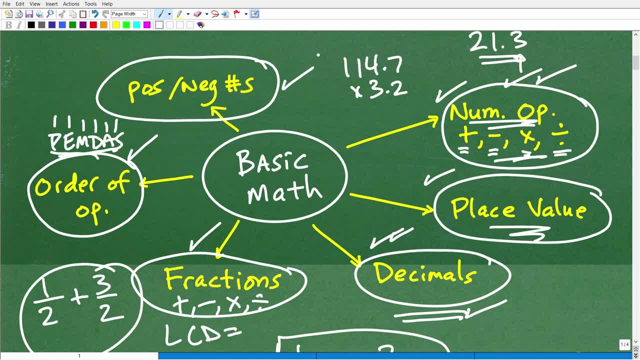 So you've got to know how the rules of positive and negative numbers, how to add or subtract, multiply and divide positive negative numbers. So, for example, let's do something real quick down here: If I said negative seven times a positive two, 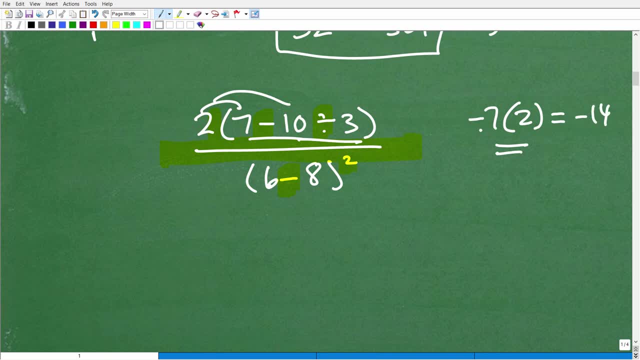 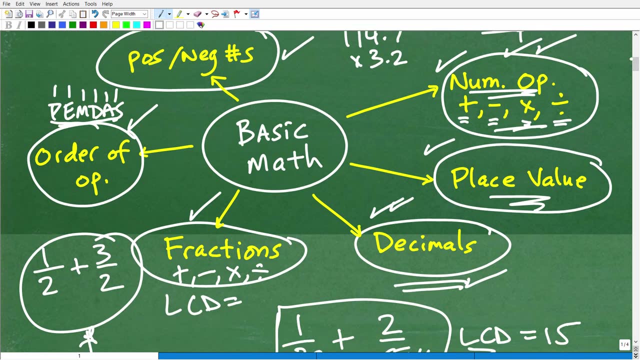 Well, this is multiplication. The answer is negative 14.. All right, A negative times a positive is a negative. So all these rules- I would say this right here- would give if somebody knew this. All right, And a particular adult was reviewing mathematics. 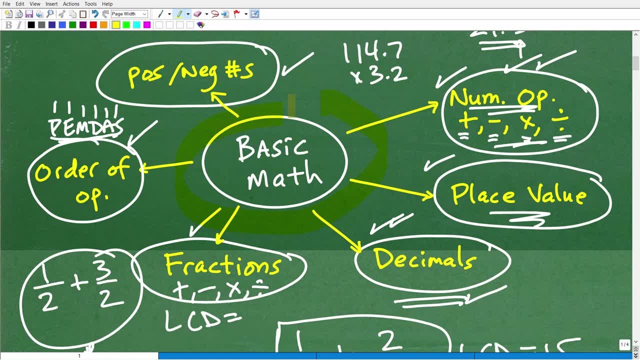 If you understood all of this really, really well, then you have a real strong, foundational kind of math toolkit to build upon. OK, one you're going to be. I think it's just, life is going to be easier for you. You're going to be able to understand, you know, the information around you. 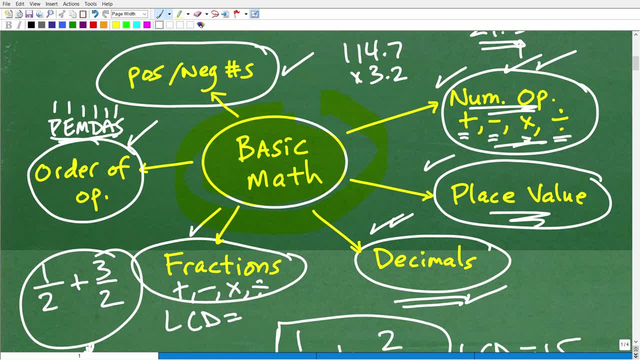 And, by the way, in this particular math course that I have this math foundation course, I go into other subjects as well, like Venn diagrams, percent, a couple other stuff. Really, the purpose of this course that I've created is to cover, to strengthen your foundations. 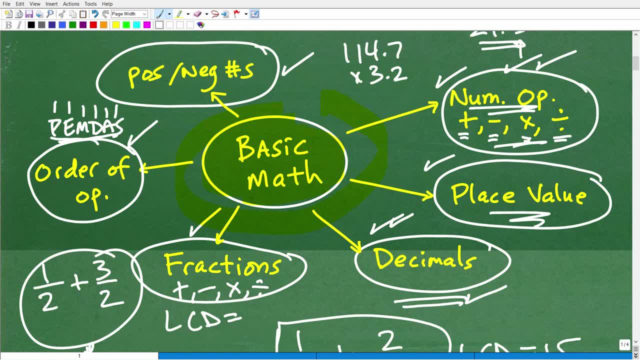 One. OK, because a lot of these things that I'm talking about are also classic weak areas for math students. OK, so when students are, let's say, in an algebra course and are having difficulty. but I've found over decades of teaching mathematics: 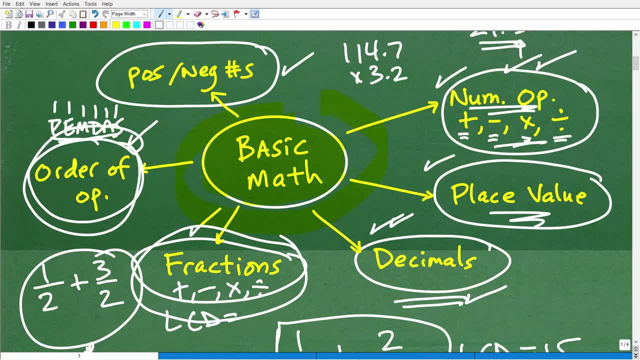 they're still a little shaky. They don't understand order of operations as well as they think they do. They still make mistakes with the positive and negative numbers. So if you have any intention on taking any kind of algebra course, you know if you strengthen or you really master all these skills. 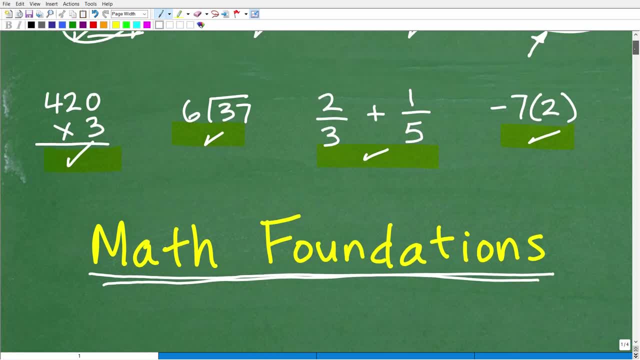 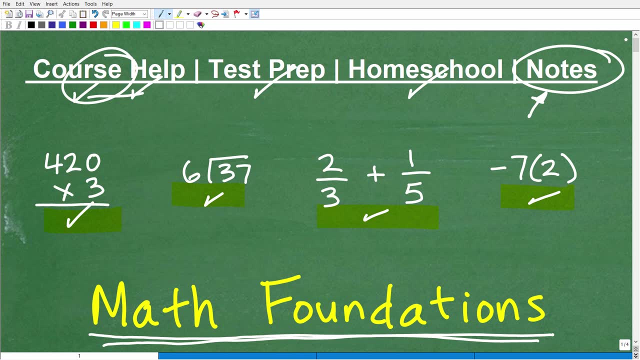 everything is going to be much, much smoother from there. OK, so that's my little take on basic math foundations. Whether you continue, continue your math education beyond this level, That's totally up to you. But if you were able to really truly master all these skills that I talked about now, I'll tell you that's pretty good. 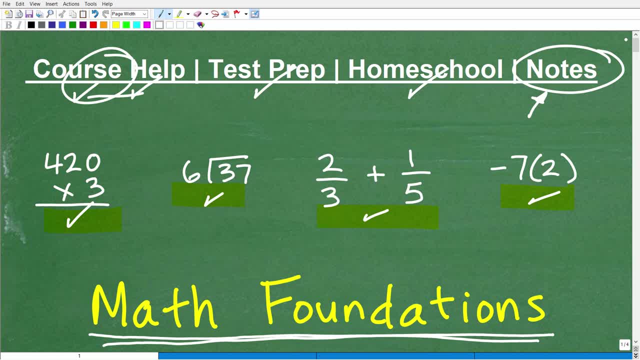 OK, there's a lot of students in you know algebra that don't even have those skills mastered. So again, if you're interested and really kind of up in your basic math skills, you might want to check out my math foundations course.